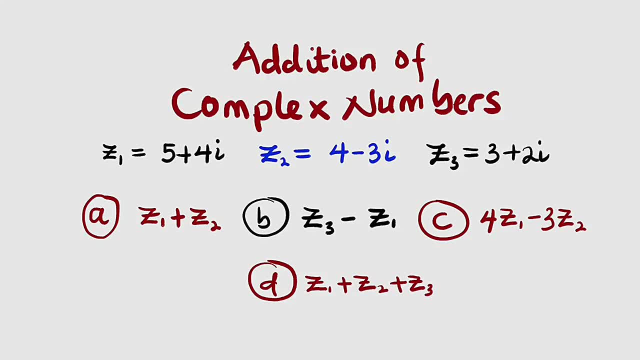 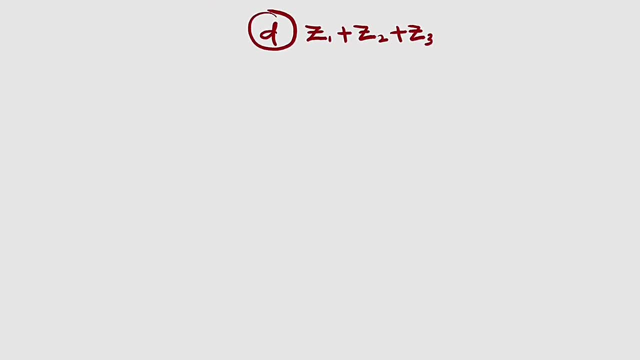 Hello, good day viewers. In this tutorial we are going to learn how to add or subtract complex numbers, But before we start let me illustrate something here. Suppose we have a complex number- z1- equal to a plus bi, And we have another one, z2, which is equal to c plus di. 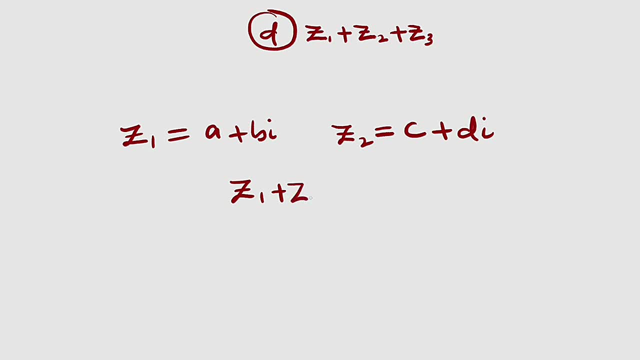 How can we add z1 and z2 together? That is the question. To add them together, you are going to add their real parts separately and also add their imaginary parts separately. The same thing for subtraction: You subtract the real parts separately, then you subtract the imaginary parts separately. 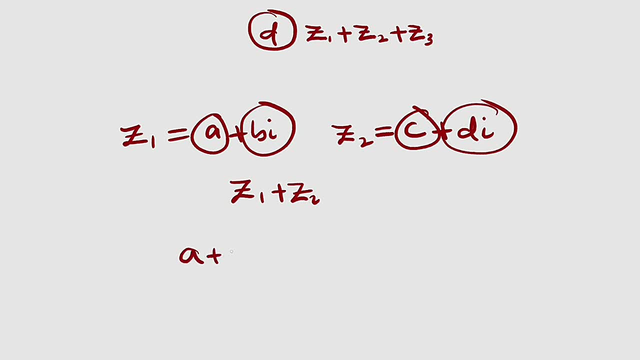 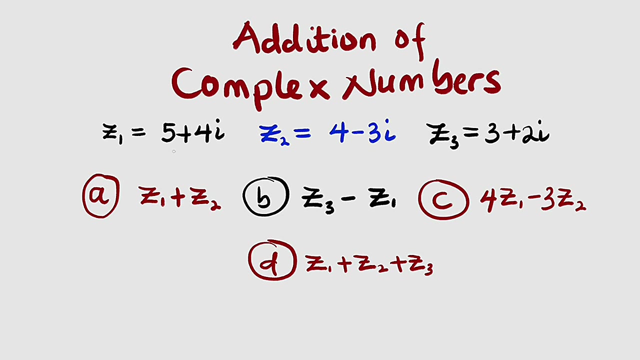 So this is the same thing as saying a plus c, then also plus bi plus di. So this is exactly how We are, given that z1 is equal to 5 plus 4i, z2 is equal to 4 minus 3i, z3 is 3 plus 2i. 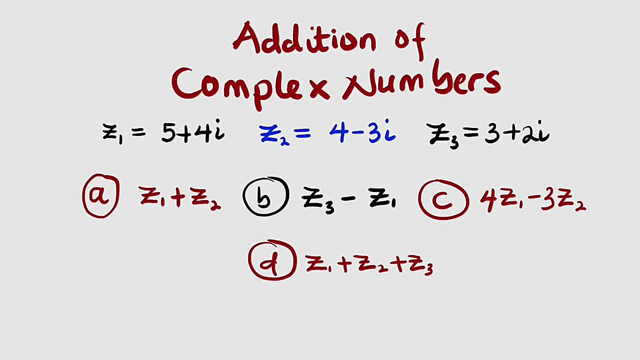 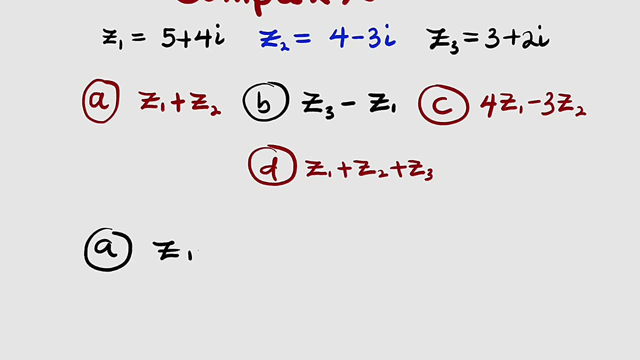 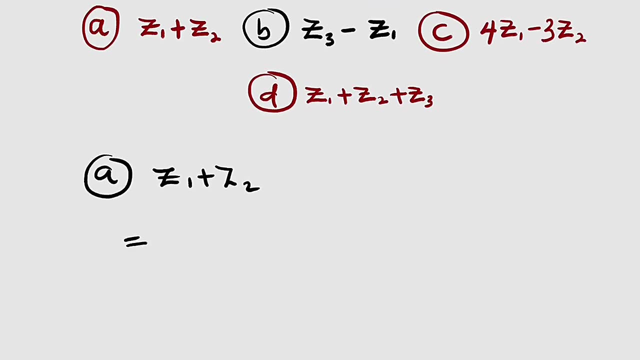 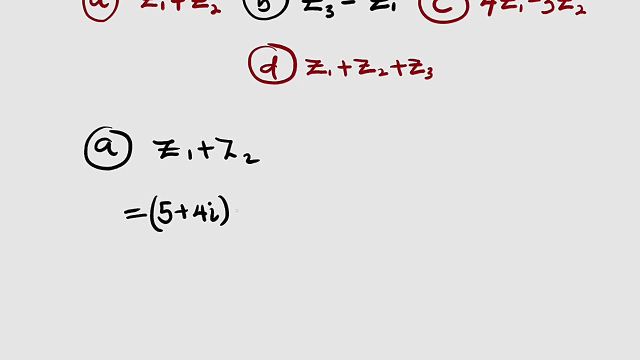 A. We want to add z1 and z2 together. So that is the first question. So a part: z1 plus z2.. You know this is equal to what is z1? z1 is 5 plus 4i, 5 plus 4i, then bracket, then plus z2, 4 minus 3i, 4 minus 3i. 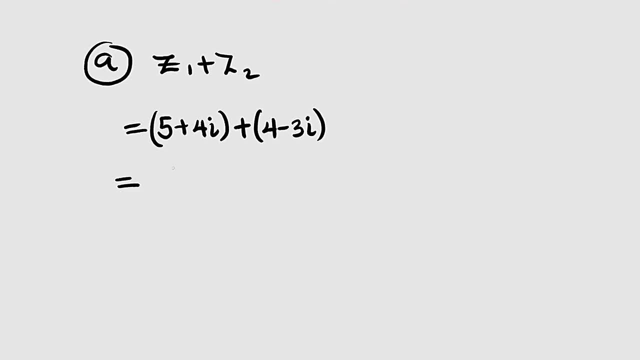 So let's collect the like terms together. This is the same thing as 5 plus 4,. right, That is the real parts. Then the imaginary parts, we have 4.. Plus negative 3, which is the same thing as 4i minus 3.. 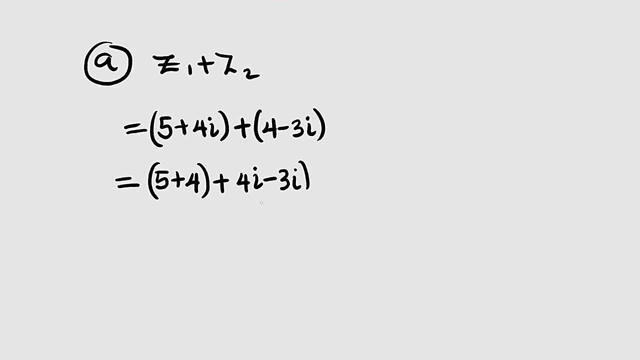 You know, negative will overpower that positive sign. 5 plus 4 is 9, then 4i minus 3i is just i. Therefore, if you add z1 and z2, you are going to obtain 9 plus i. 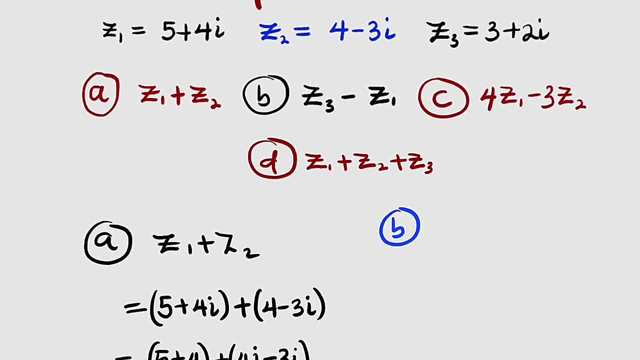 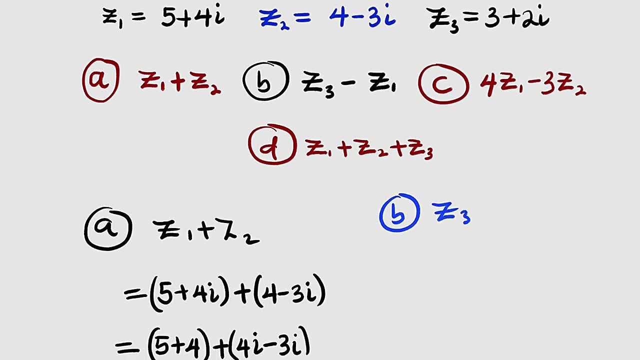 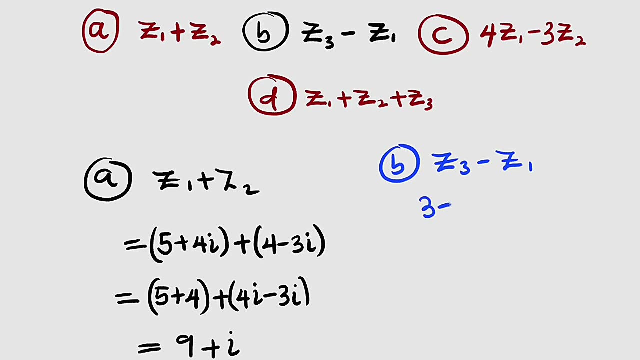 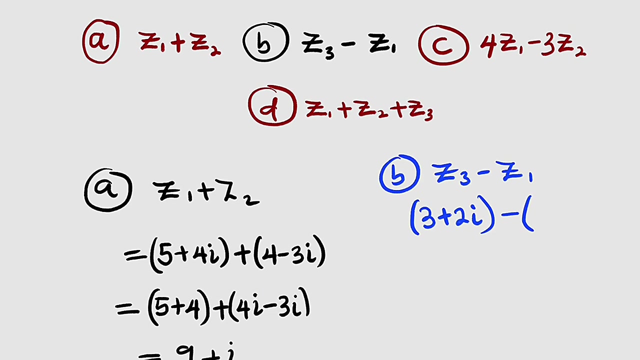 Then what about the b part? The b part? We are asked to subtract z1 from z3.. z3 is 3 plus 2i, so we have 3 plus 2i, the whole of this minus What is z1?. 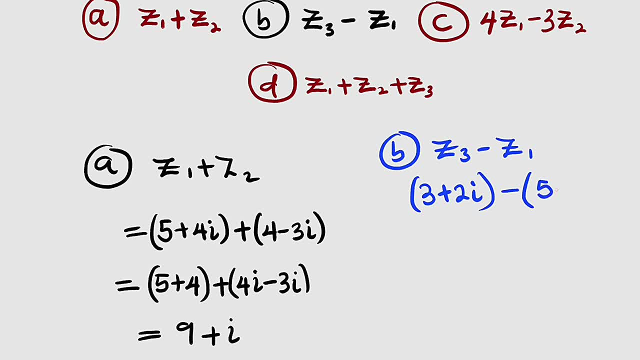 5 plus 4i. 5 plus 4i. First of all, we have to distribute z1 and z2.. What is z1?? 5 plus 4i. 5 plus 4i. First of all, we have to distribute z1 and z2.. 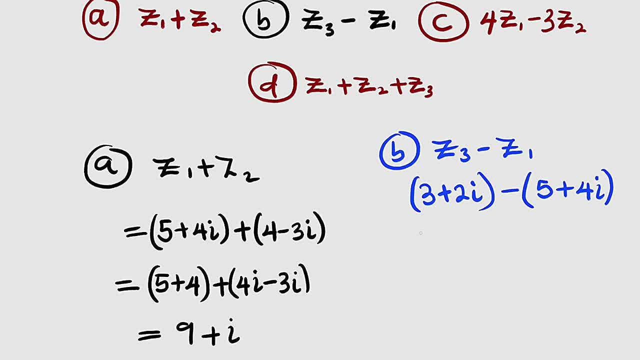 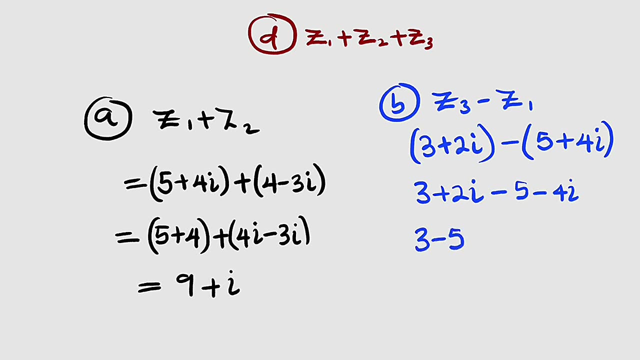 We have to distribute this negative sign into the other parenthesis. So, to the left hand side, we still have 3 plus 2i, then minus 5.. Then minus 4i. So let's collect the like terms. We have 3 minus 5, which are the real parts. then we have plus 2i, which is this one, and 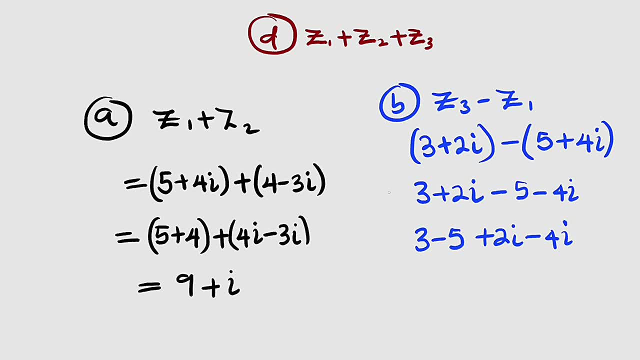 the other one is minus 4i. 3 minus 5 is negative 2, so we have negative 2 here. then 2i minus 4i is also negative 2i. so this is the solution to this problem: z3 minus z1 is exactly negative 2 minus 2i. then. 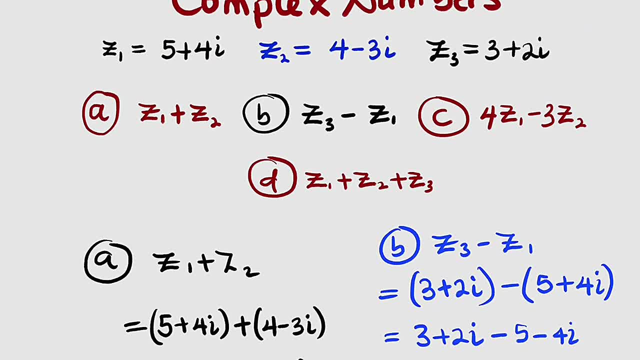 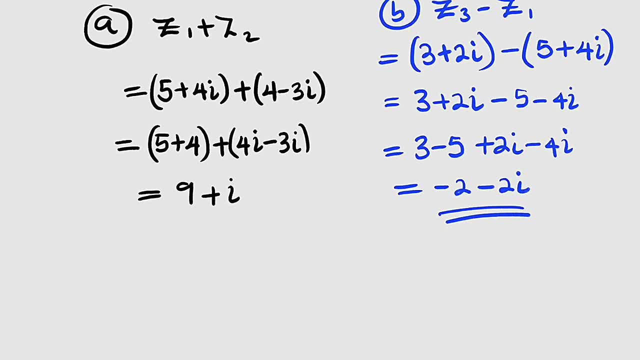 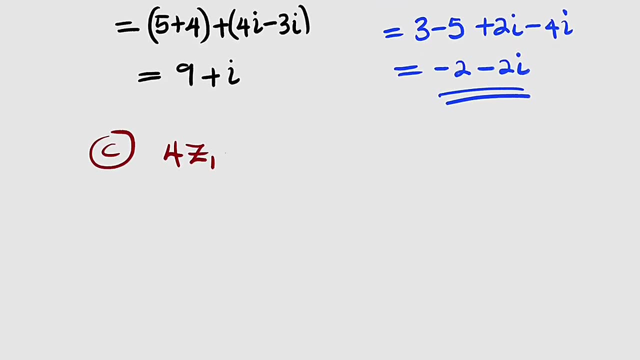 let's take the C part. the C part we are asked to evaluate or simplify: for z1 minus three, visit two. so the CPAT foeth at one minus three, that two minus three is it two. this is the same thing as four multiply by the whole of that one and that 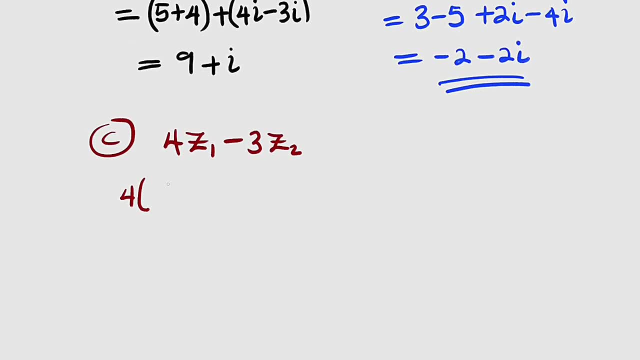 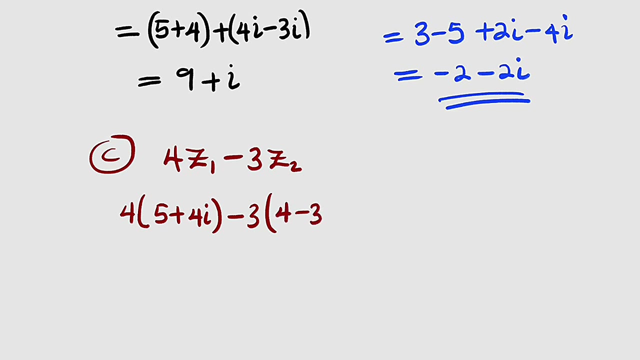 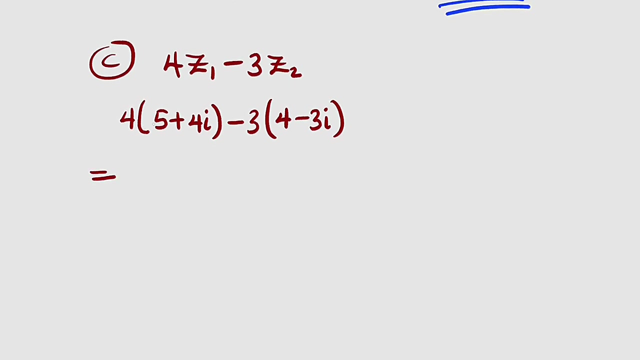 one is five plus four, I, five plus 4i. the minus 3 X Multiplies by Z2, which is 4 minus 3i, 4 minus 3i. So now let us expand the parenthesis. first The left-hand side we have: 4 times 5 is 20 plus 4 times 4 is 16i. Then the other. 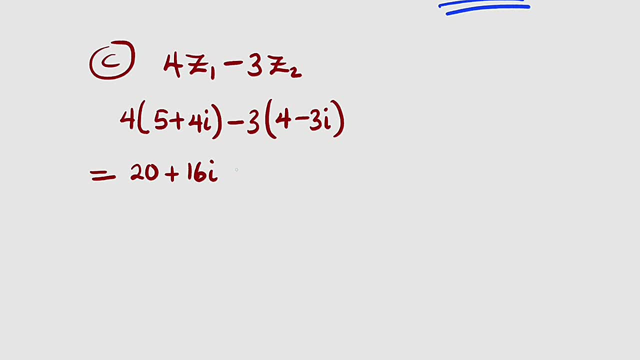 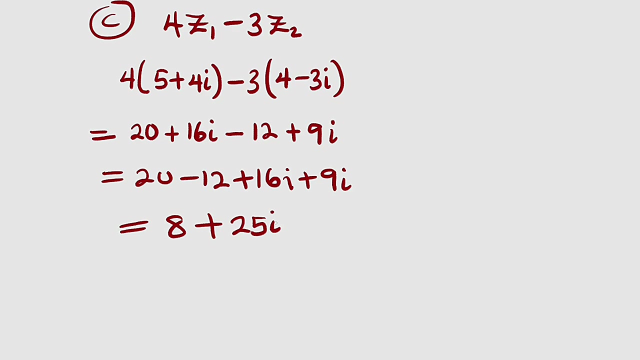 parenthesis: negative 3 times positive. 4 is negative. 12, negative negative is positive 3 times 3 is 9i. So we collect the like terms. We have 20 minus 12, then plus 16i plus 9i. 20 minus 12 is 8, plus 16i plus 9i is 25i. Hence simplify it. 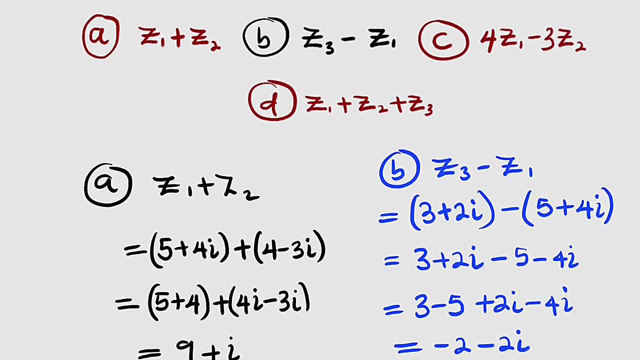 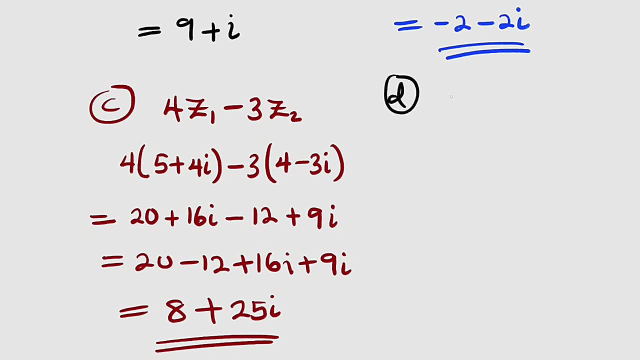 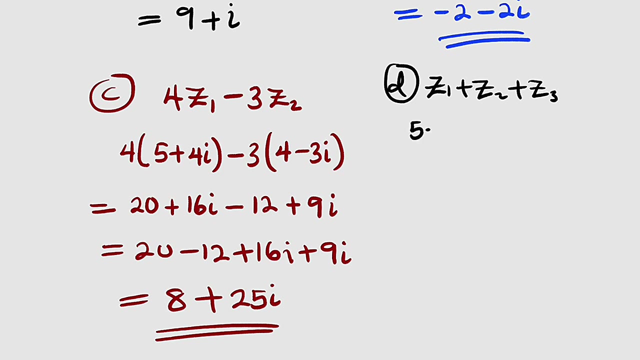 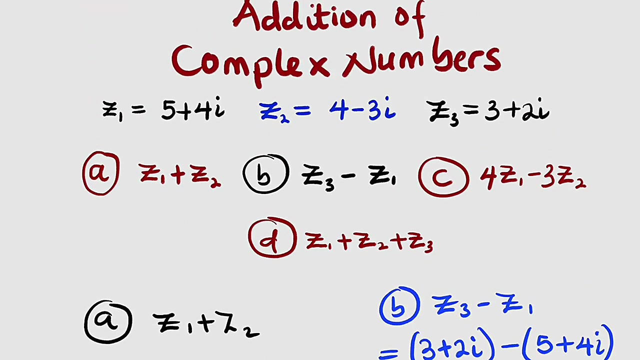 Then the last one, which is the part. it's stated that we should add all of them together: Z1, Z2 and Z3. So we have the part Z1 plus Z2 plus Z3. What is Z1? 5 plus 4i, 5 plus 4i, Then Z2, 4 minus 3i. 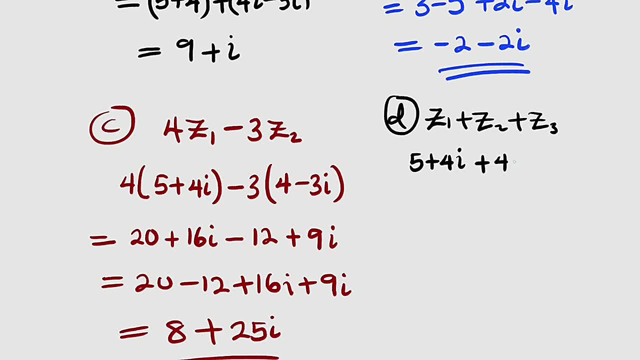 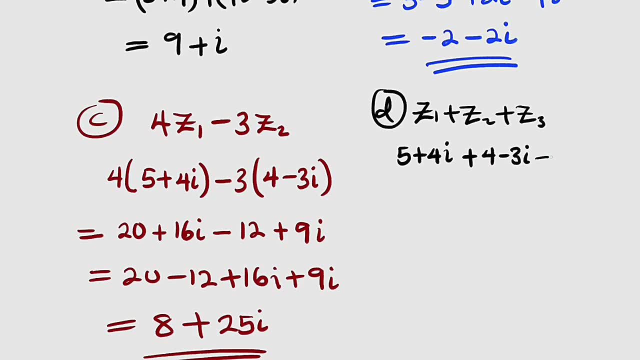 3i plus 4 minus 3i. Then the last one, Z3, 3 plus 2i. 3 plus 2i. Collect the like terms. We have real, real and real together. let's add them, We have 5 plus. 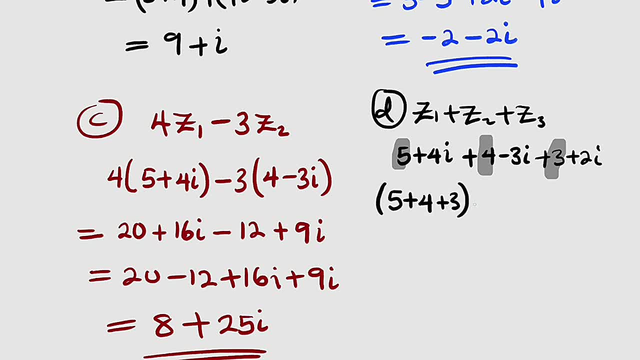 4 plus 3 separately. then plus the other parts, i minus 3i plus 2i. The left hand side- we have: 5 plus 4 is 9 and 9 plus 3 is 12, so we have 12 here. Then plus the imaginary parts, we have 4i minus 3i, which is just. 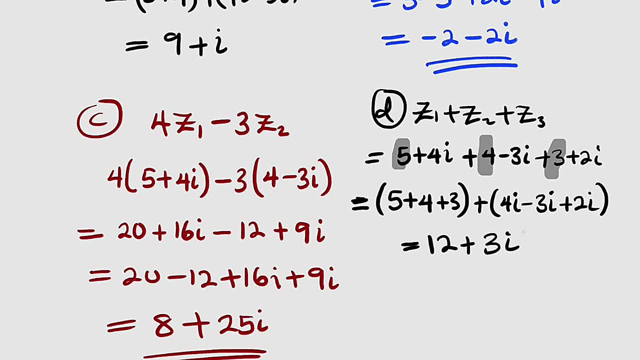 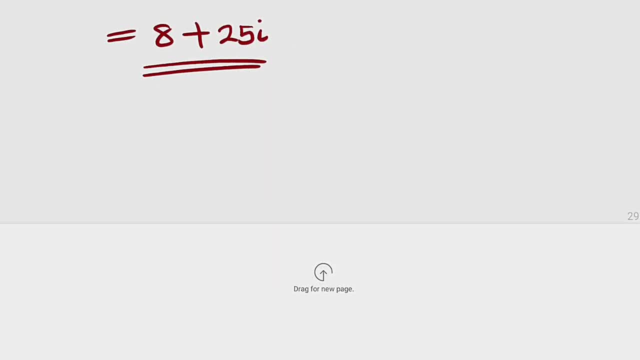 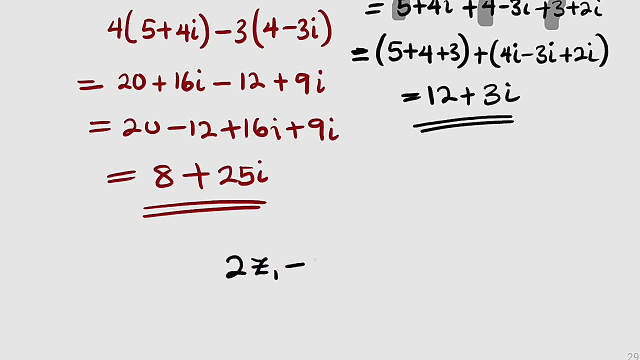 i and i plus 2i is 3i, so we have 3i here. So this is the solution to z1 plus z2 plus z3.. So let me give you an assignment. I would like you to evaluate 2z1 minus 3z3.